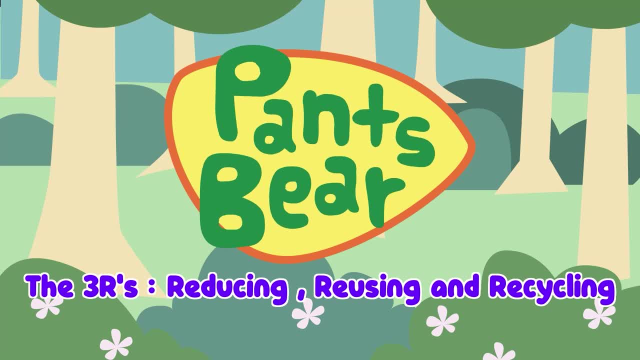 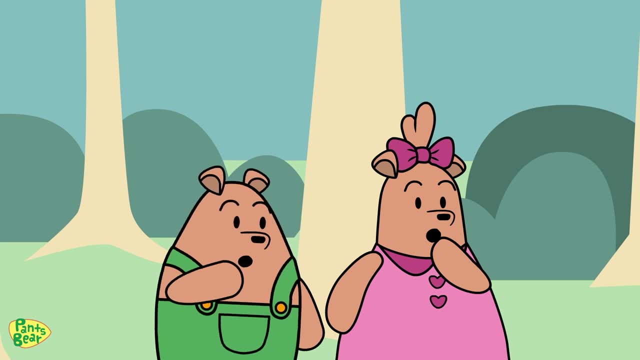 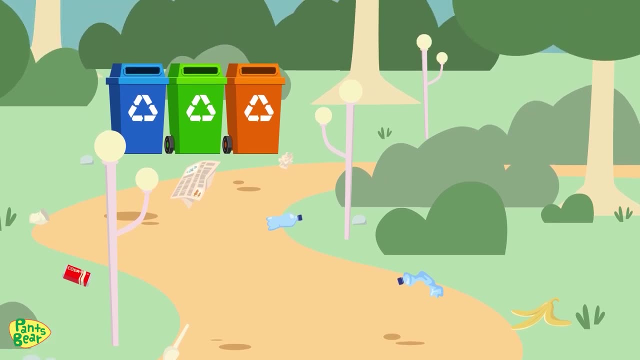 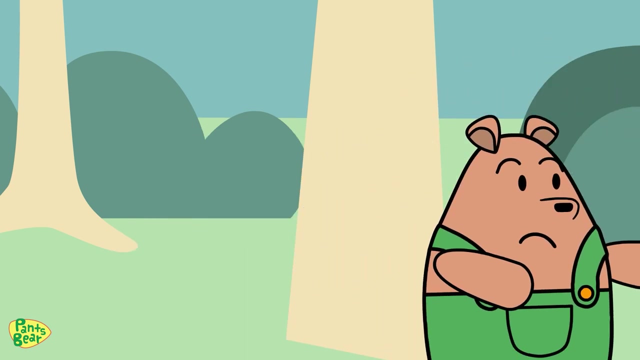 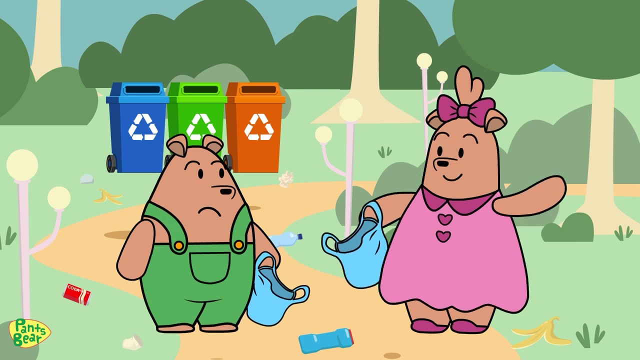 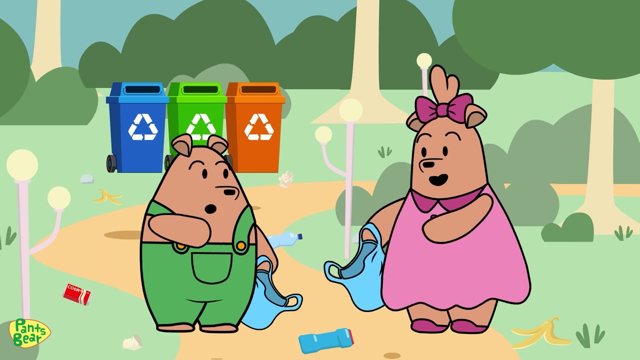 The three R's: Reducing, Reusing, Recycling. Wow, look at all this trash. What a mess Pants Bear. We have to clean this up. What are we doing? We're reducing, reusing and recycling. It's important to keep our environment clean and take care of our planet. 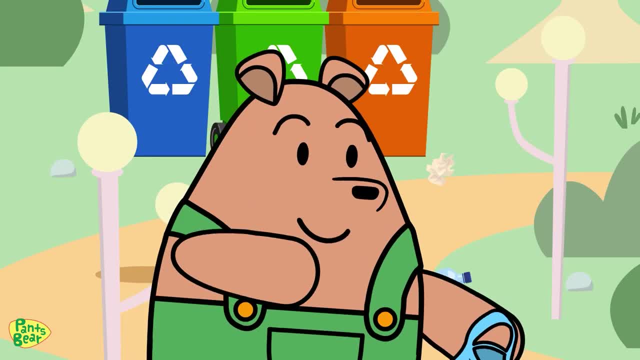 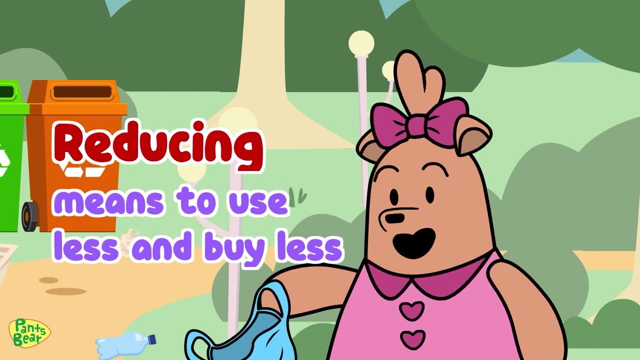 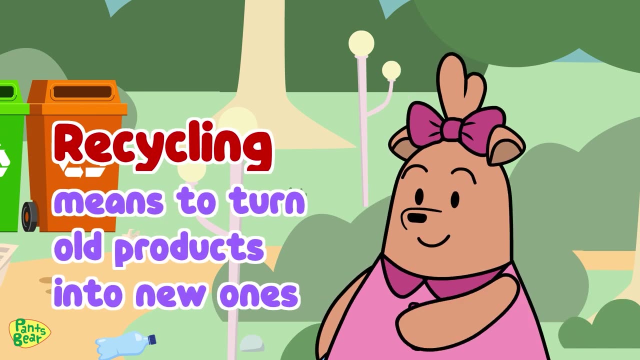 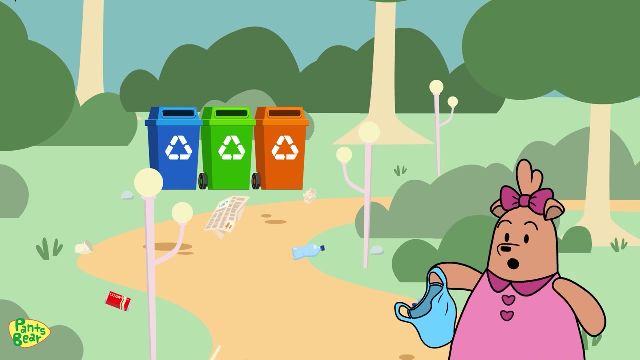 What does reduce, reuse and recycle mean? Reducing means to use less and buy less, Reusing means to use things more than once, And recycling means to turn old products into new ones. All sorts of things can be recycled. Some of the most common processes used today recycle. 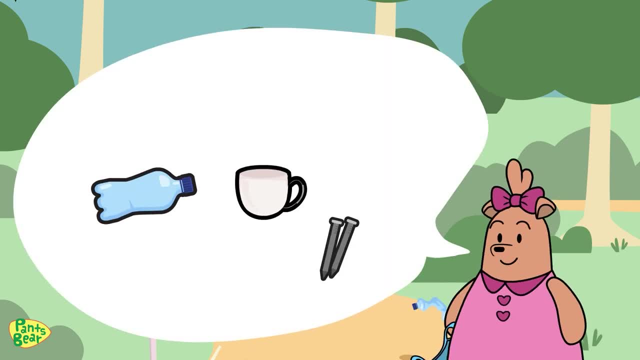 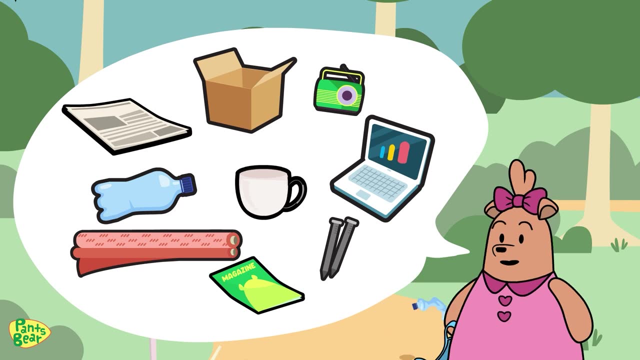 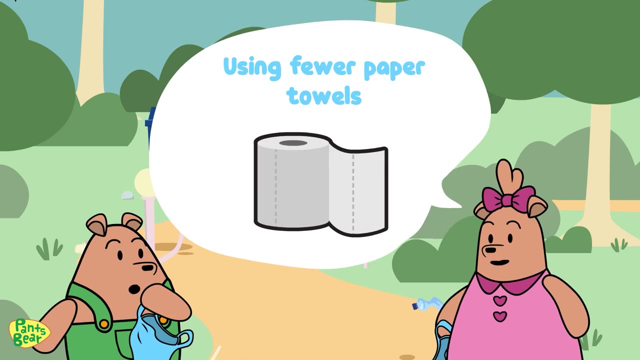 plastics, glass, metals, electronics, computers and accessories, textiles, newspapers and magazines, cardboard. How can I recycle? How can I help? Recycling does not have to be difficult. You can help by using fewer paper towels, bringing your own reusable water bottle. 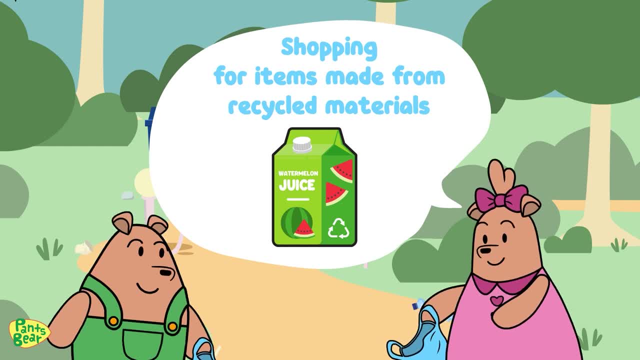 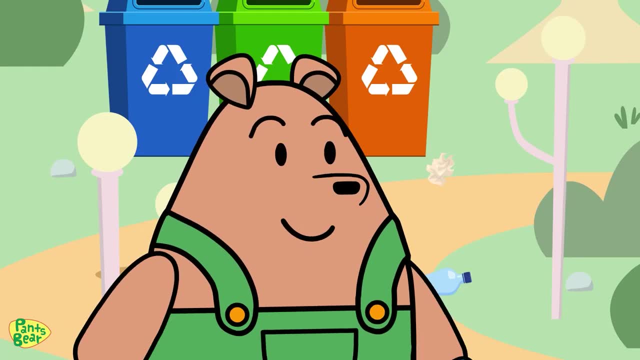 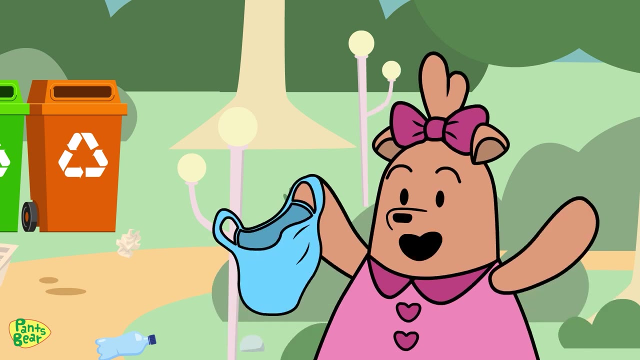 and shopping for items made from recycled materials. I'm so glad we're doing this- Me too. Recycling is vital for many reasons that affect the future of all children. Recycling is vital for many reasons that affect the future of all children. This is the only planet we have. 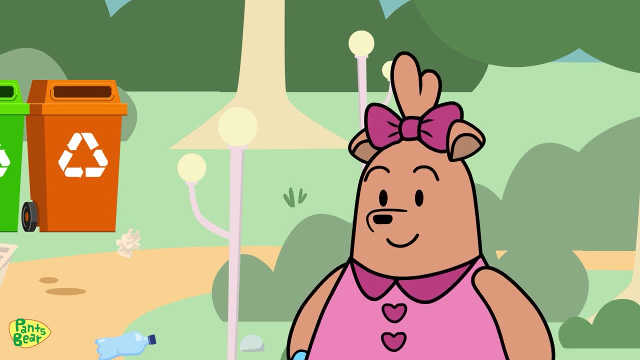 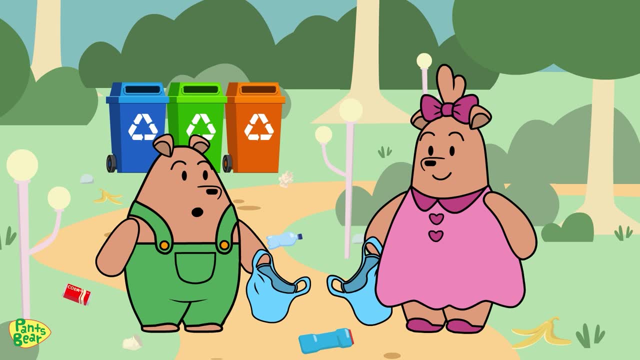 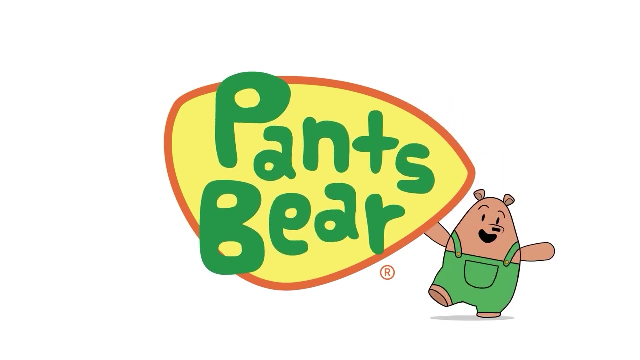 so it's important to do our part and keep it clean and healthy. Wow, I've learned so much from this experience. I'm really excited to reduce, reuse and recycle from now on. Goody Goody.